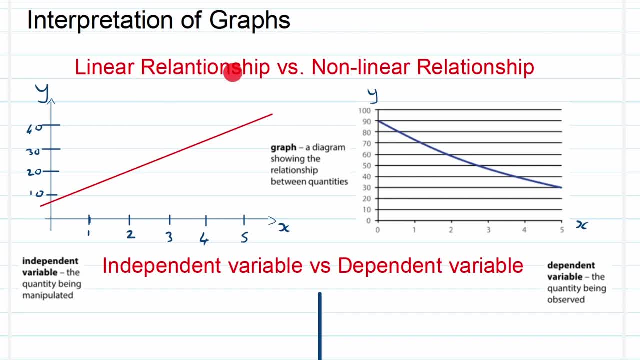 terminologies right: Linear relationship versus a non-linear relationship- And if you think carefully, it's exactly what it says. Is there a linear relationship between two quantities? The first quantity we would refer to is the independent variable. So what is the one that you choose? Let's say you choose a value of well, x, in this case. 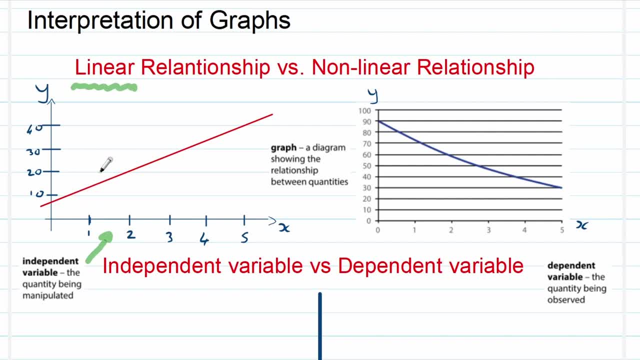 What will be the corresponding y value? Now, if the relationship between the x and the y is a straight line, then we call it a linear relationship. So this has to be a straight line for it to be linear. Okay then, a non-linear relationship. 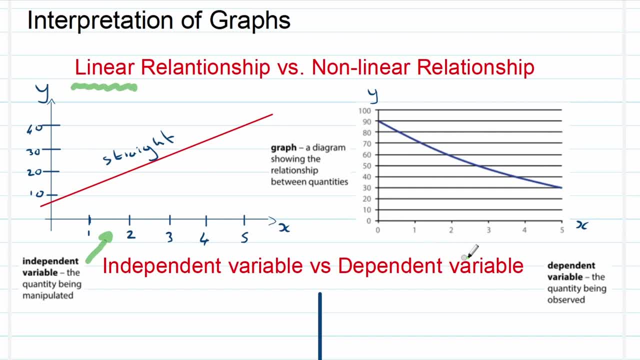 Is exactly again the same thing. We are looking at the independent variable, the one that you choose, versus the output value, the dependent variable, And if the relationship is not a straight line, then we call it a non-linear relationship. So it's very important. 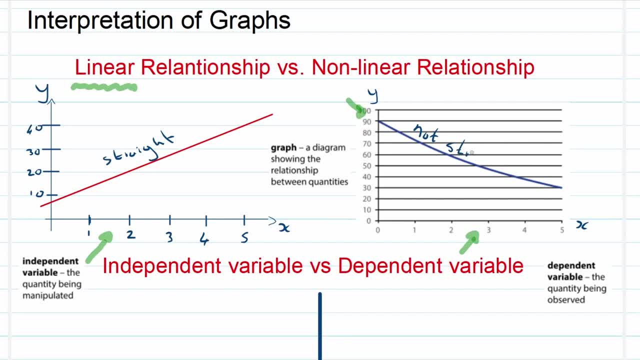 to remember. not straight means non-linear, Straight means linear. Okay, then, the second concept I would like to explain is the difference between an independent variable and a dependent variable. So independent variable is a quantity being manipulated. Now, for me this is a little bit vague. I would like to clarify. This is the one that I would say. 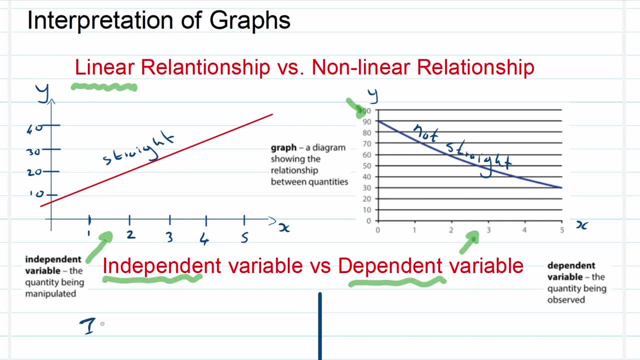 this is the input value. okay, So this is the one that you are choosing input. So I'm saying, okay, let's take this as time like one, two, three, four and five minutes, And the 10,, 20,, 30 and 40 is the amount of jelly beans. 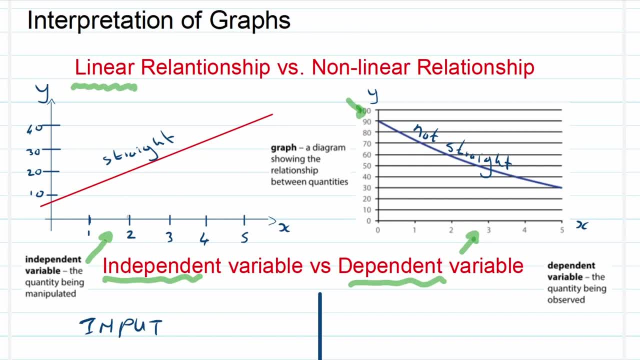 being thrown into a bucket. The input value is: I want to know, okay, in two minutes, how many jelly beans has been thrown into the bucket. Now, according to this graph, it's 20.. Okay, so you can see. the input value is: I'm asking at this amount of time. 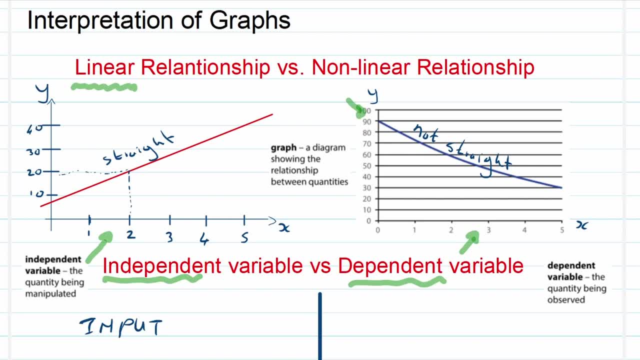 two minutes, and then the output value, which is the dependent variable. the output value will then be my answer: no, in two minutes there's 20 jelly beans in a bucket. so the output is dependent on the input, which is independent. that's why they say the quantity being manipulated, in other words i. 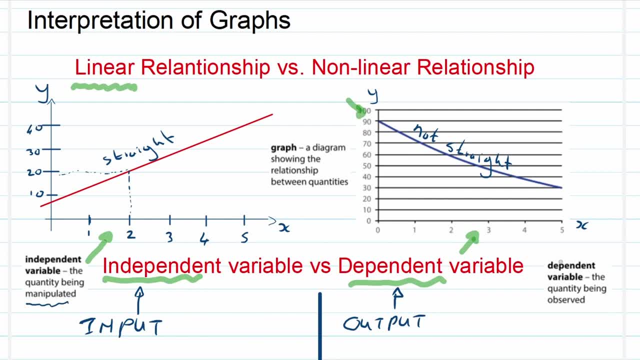 i am choosing my input value, then the dependent variable is the quantity being observed. now, that is my answer. why do i get out so the same year with any graph? let's say this is also a representation of the amount of jelly beans into a bucket at two minutes we know. in this specific case we can read it off the. 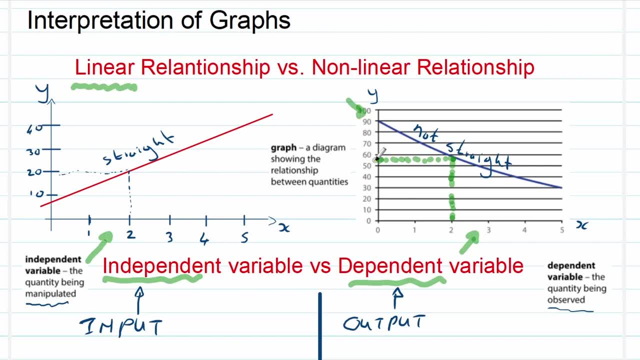 graph. the answer is about 60- 65.. so you understand. so is independent, and that's normally the one on the x-axis. That's the one that's independent. That's where you put it. Always put your independent variable on the x-axis, Your dependent variable. 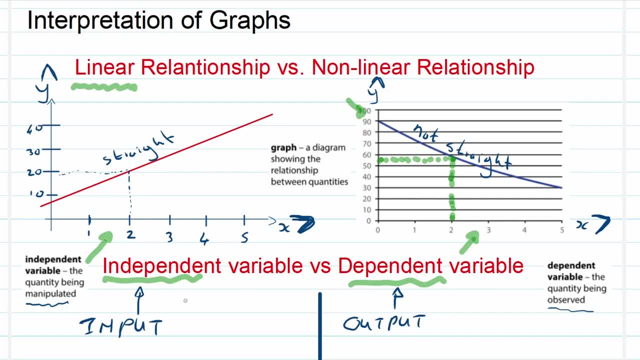 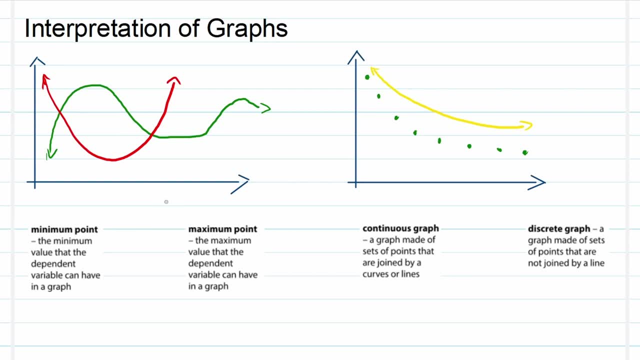 you put on the y-axis, That means the vertical axis. Hopefully this is clear. Let's look at the second part of this video, Minimum and maximum point on the graph. Now, if you observe over here the green graph, you can see its highest output value, The highest y value, right over there. 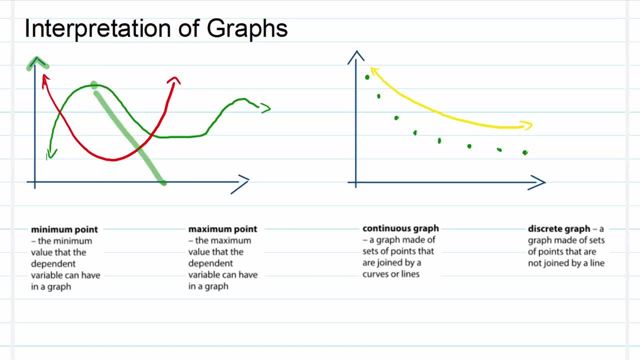 That is the highest we'll go. That's the maximum point. Whenever we look at a maximum and minimum point, we always look at the output value, That which is on the y-axis. Okay, so maximum point is the maximum value that the dependent variable can have in the graph. So remember your dependent. 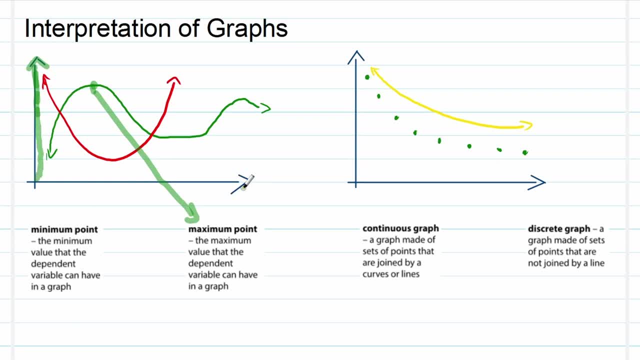 variable Is on the y-axis, Your independent variable is always on the x-axis. Now, the same here with the minimum point. You can see that's the lowest output value. That's right over here and that's our minimum point. So the minimum value that the dependent variable can have in the graph. So this: 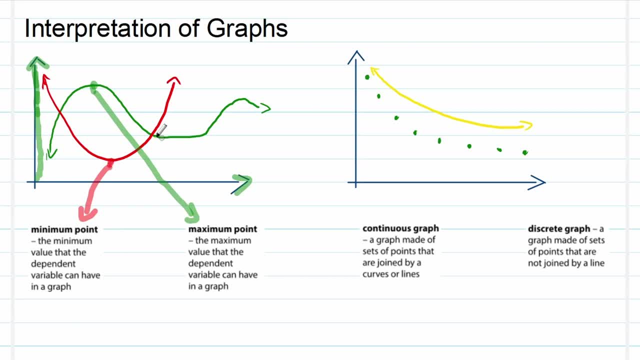 is a good example where it's relevant. You can see, for the green graph, this is a local minimum, but that value is still lower. So we don't really have a minimum value. So we can see that the minimum is higher than the minimum. The same for the red graph: We don't have a maximum, It will just go on. 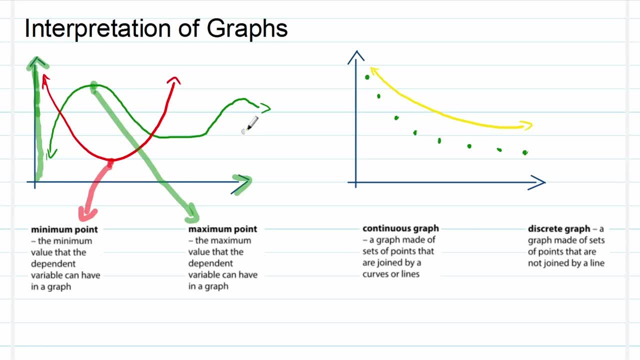 having a higher value increase as the dependent, the independent value increases. So this is the difference between a minimum and a maximum point. And thirdly, let's look at what a continuous graph is and what a discrete graph is. Continuous is exactly what it says. A continuous graph is a graph. 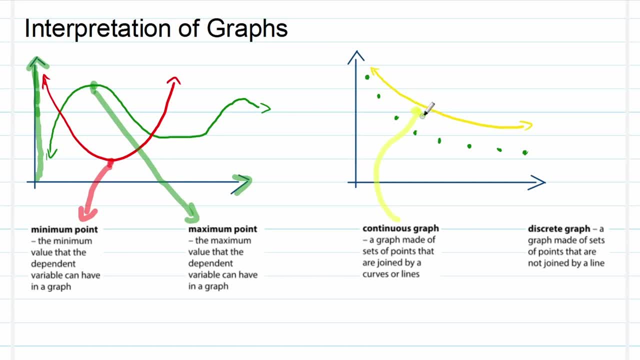 that continues like the yellow one. You can see it just continues. It continues like the yellow one, It continues, It doesn't stop. There's no break in the graph. So it's a graph made of a set of points that are joined by a curved line. So the moment you see a line like this, then you know it's. 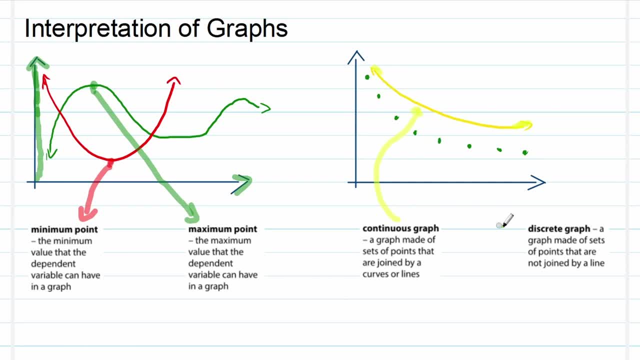 continuous. But, on the contrary, if you look at a discrete graph, it's a graph made of a set of points that are not joined by the line, Like the green graphs, All these dots, they represent a discrete graph. It's not continuous, It's a discrete graph. It's a discrete graph. It's a discrete graph. 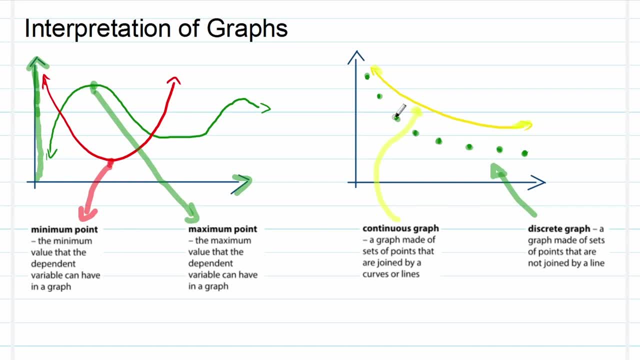 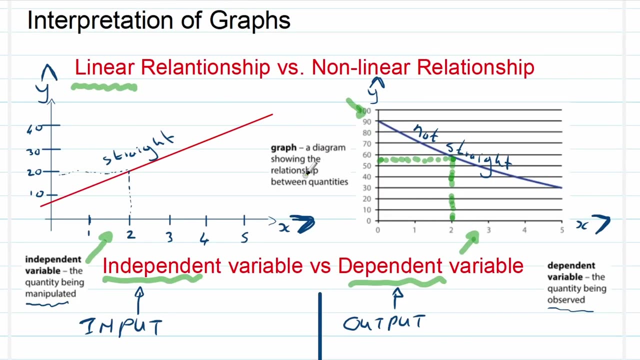 It's not continuous, It's not joined by a line, It's just the dots. That is a discrete. So here we go. These are the basic terminologies for graphs. Remember, a graph is a visual representation. Right, A graph is a visual representation that shows your relationship between quantities. 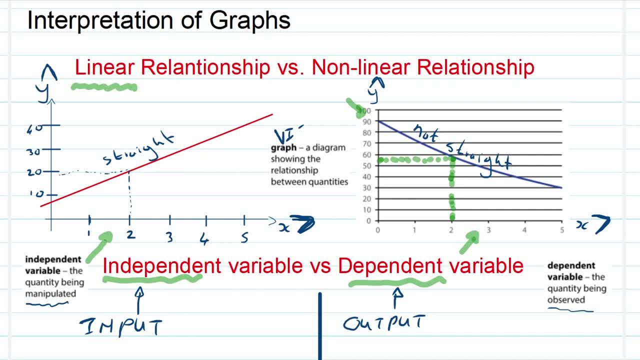 So please add here it is a visual. Okay, It's something that you see, So that will help you to remember it as well. Stay tuned for the next video on graphs, Subtitles by the Amaraorg community. 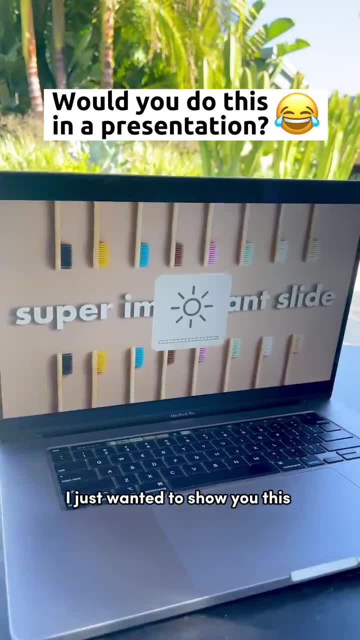 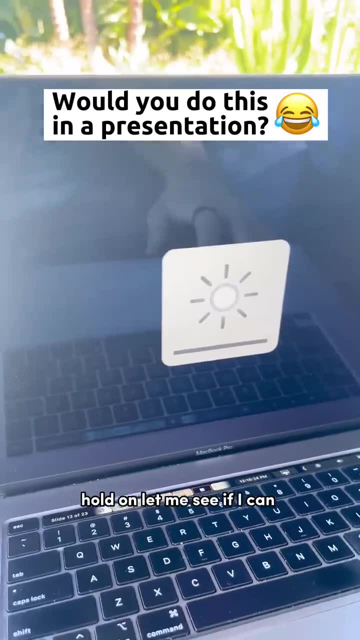 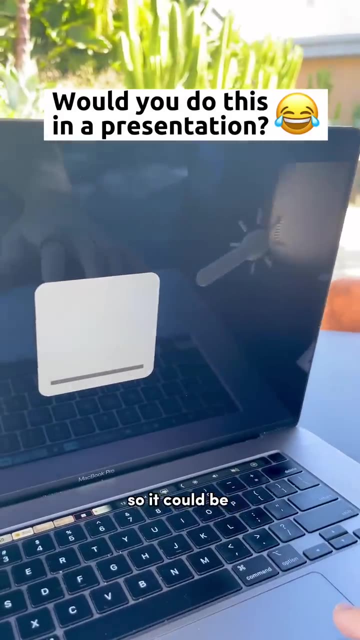 Welcome to my very important presentation. I just wanted to show you this one slide I've been working on. Oh, my computer keeps having this brightness issue. Hold on, let me see if I can find the switch. I mean, we got to be able to see the slide right, So it could be. 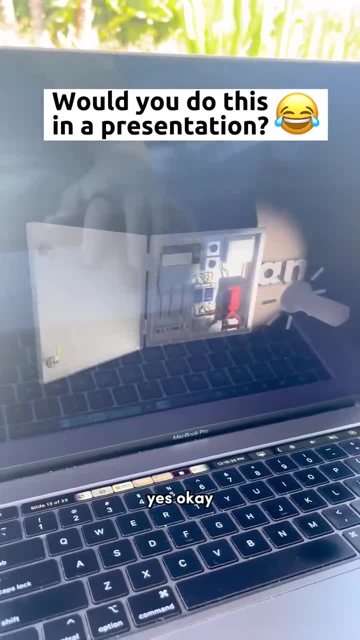 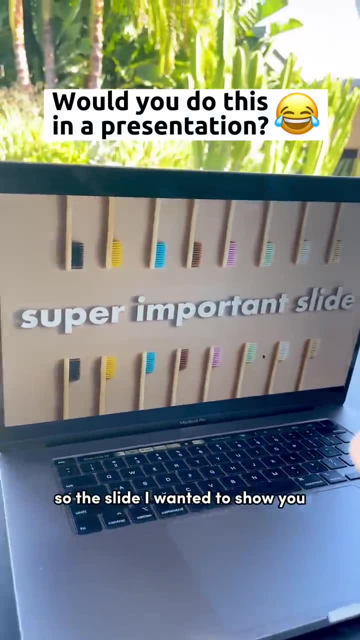 in the circuit breaker, Yes, Okay. And then the big red switch: Okay, It's always a big red switch. Okay, perfect. So the slide I wanted to show you- actually that was it. Would you use that slide?